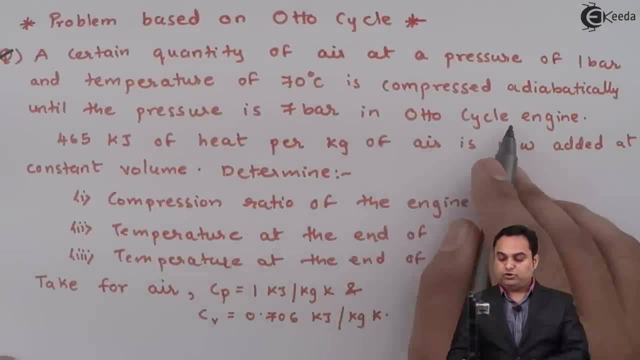 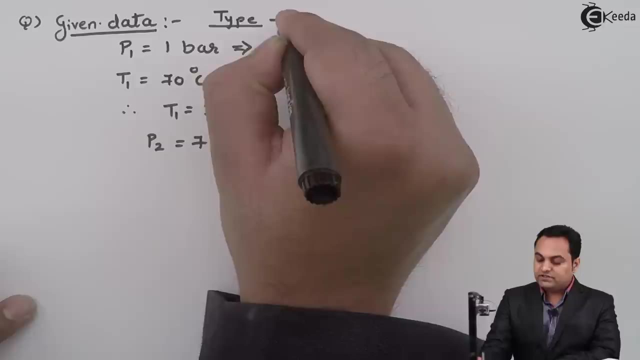 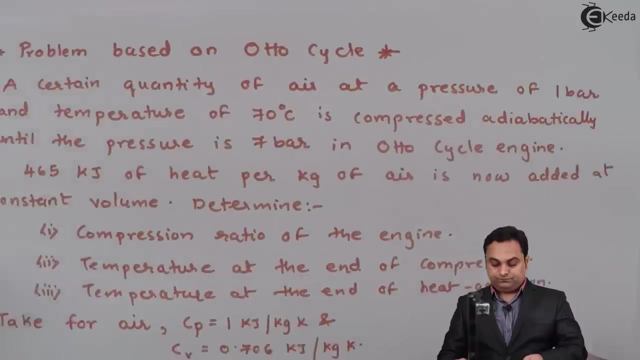 so 7 bar in auto cycle engine. so 7 bar in auto cycle engine. so here the type is given, so I'll write the type. in this case it is auto cycle. now, 465 kilojoule of heat per kg of air is now added at constant volume. 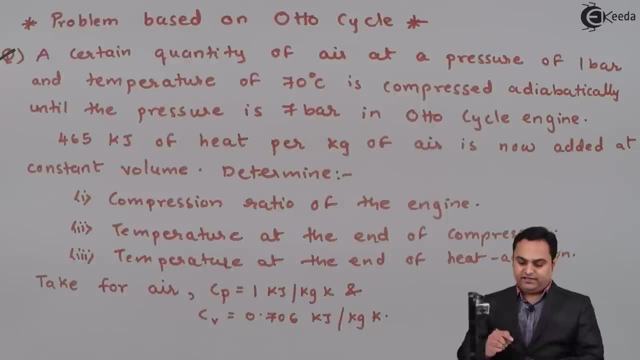 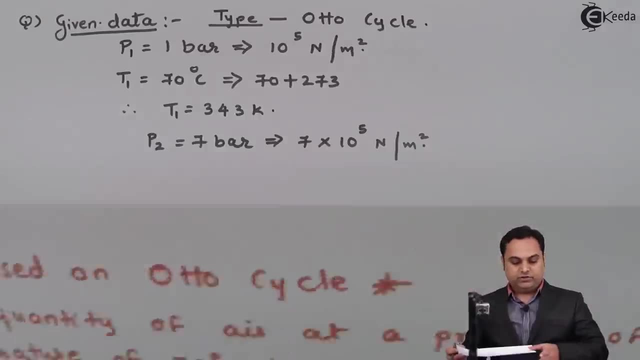 in case of auto cycle, the heat gets added at constant volume and that heat is given as 465 kilojoule and since it is on per kg basis, 465 kilojoule of heat per kg of air is now added at constant volume. so I'll write down: therefore: heat added Q suffix A. 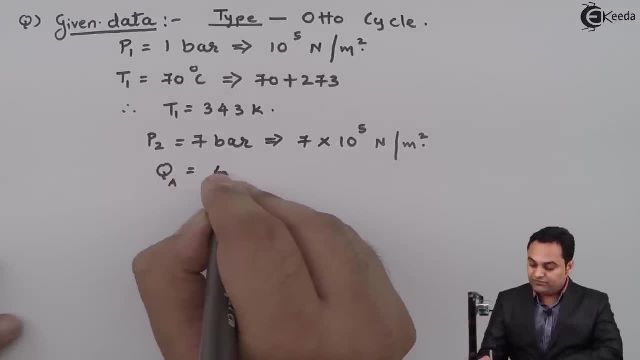 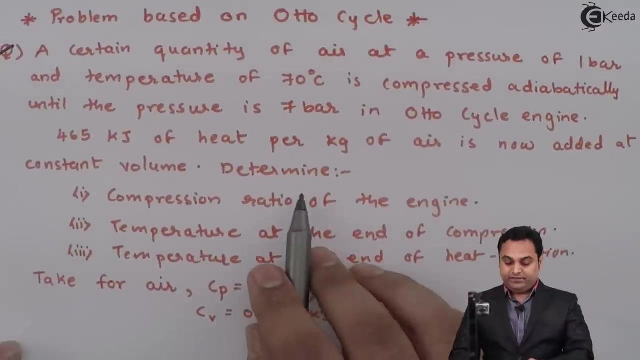 it is called as the amount of heat added, and it is 465 kilojoule per kg. so from this it is clear that here we have to take mass of air as 1 kg now determine. there are 3 questions which have been asked here. 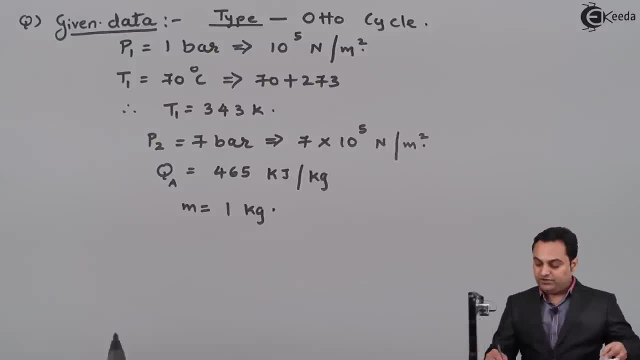 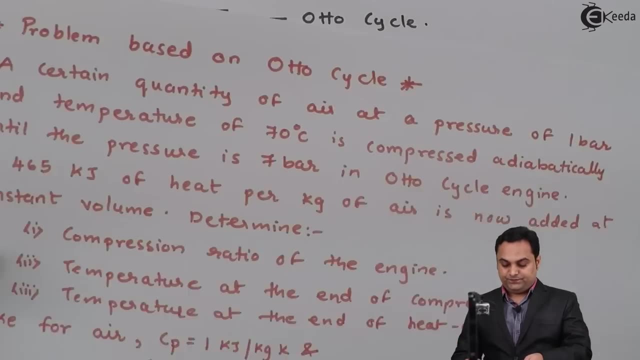 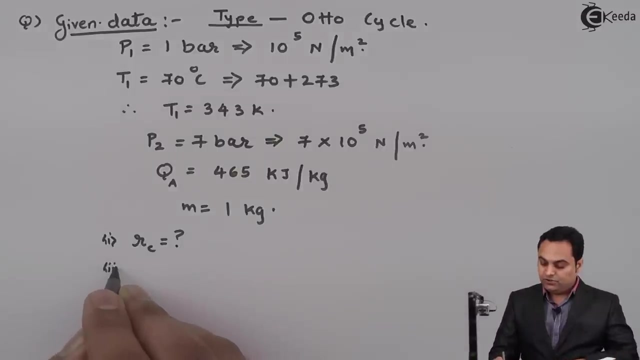 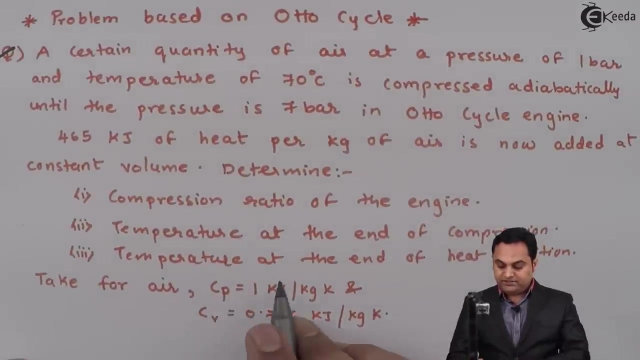 first is compression ratio of the engine. compression ratio is denoted by r suffix c. next temperature at the end of compression. so temperature at the end of compression will be t2, and then temperature at the end of heat addition. heat addition gets started at point number two. 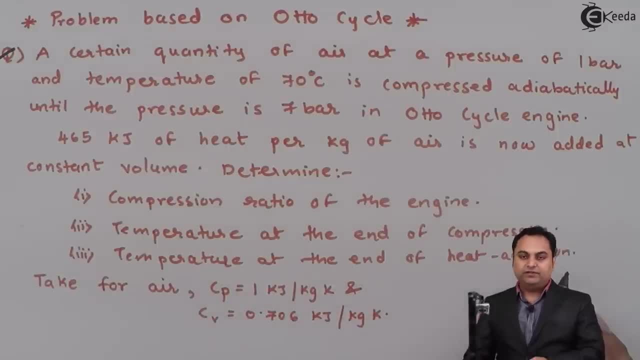 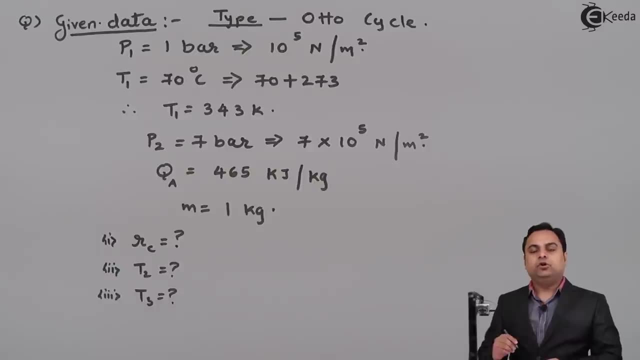 and it gets completed at point three. so temperature at the end of heat addition means we have to calculate t3 and accordingly these terms would be understood. once i start the solution, that is, in the solution part, i will be drawing the pv and ts diagram. from that we can get an idea that what temperatures are to be calculated. 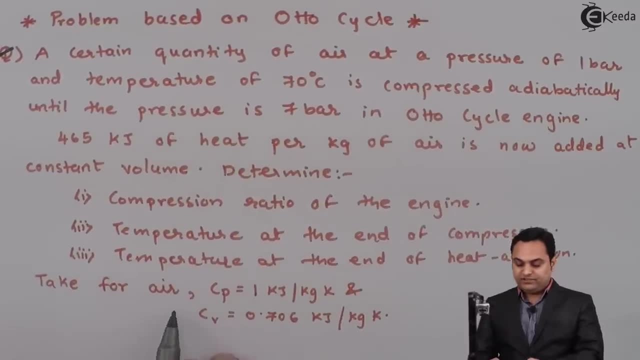 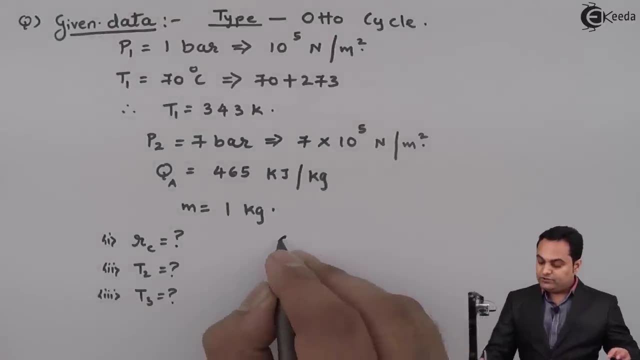 next take for air. some values are given for air. cp, that is specific. heated constant pressure is one kilojoule per kg kelvin, so cp is equal to we have to take for air one kilojoule per kg kelvin and cv, specificated constant volume, that is 0.706. 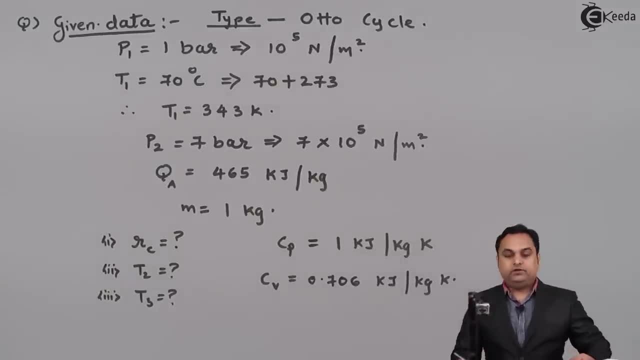 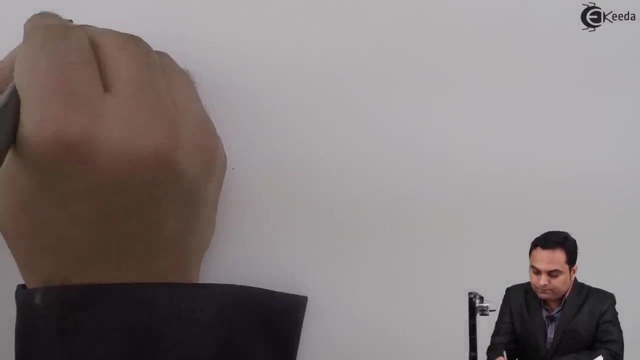 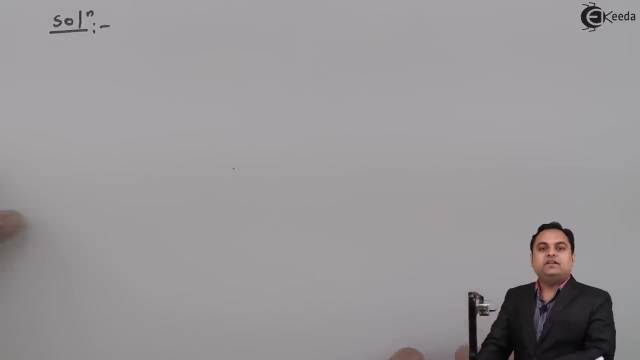 kilojoule per kg kelvin. now, with the data available to us and we have understood what are the unknowns to be calculated, let us try to get the solution to this problem now in the solution part, since it is given that here the type of cycle is auto. so for auto cycle we need to draw pv and ts. 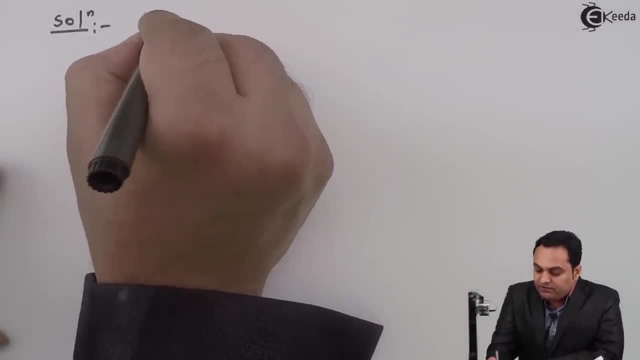 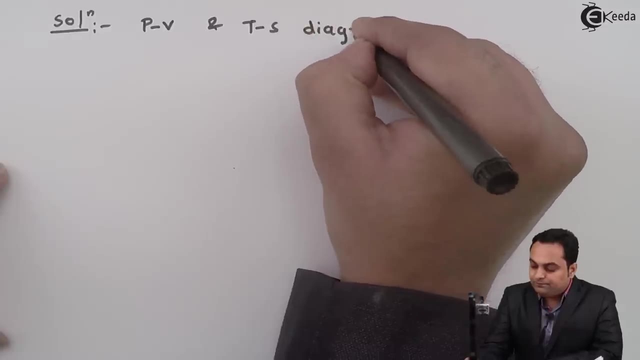 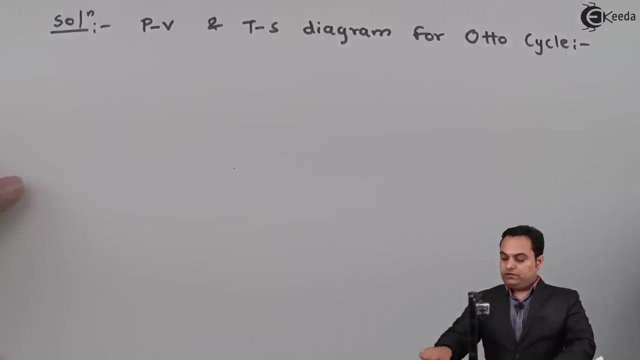 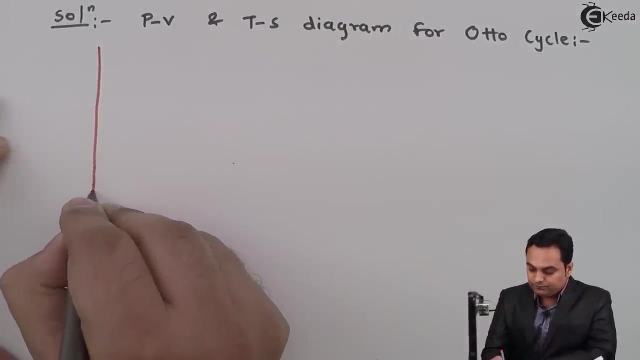 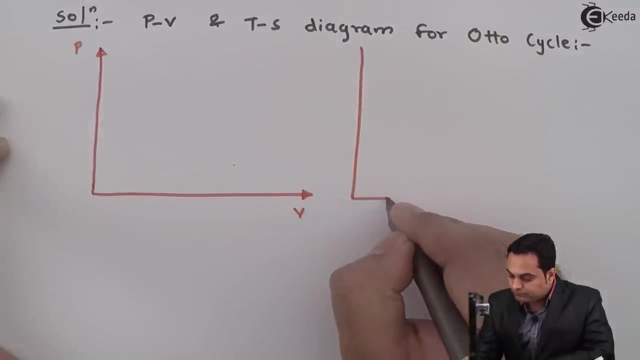 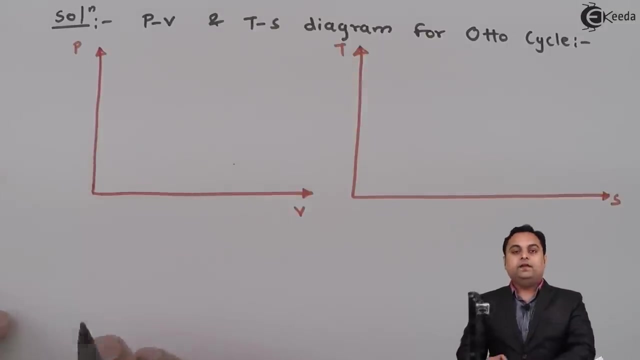 diagram. so i'll write down that. first i'm drawing pv, that is pressure volume, and ts, that is temperature entropy diagram for ultracycle. and that diagram now i'm going to draw now in the pv and ts diagram. first i'll start with pv diagram. in case of autocycle there are four. 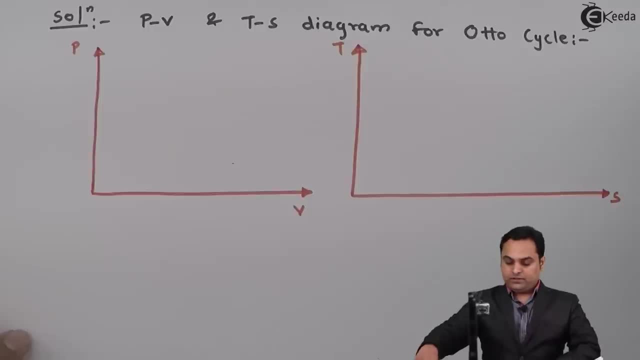 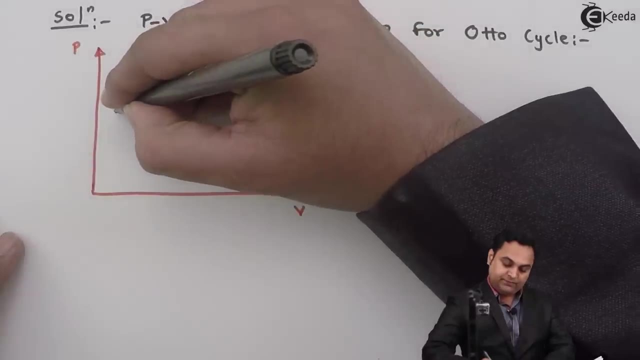 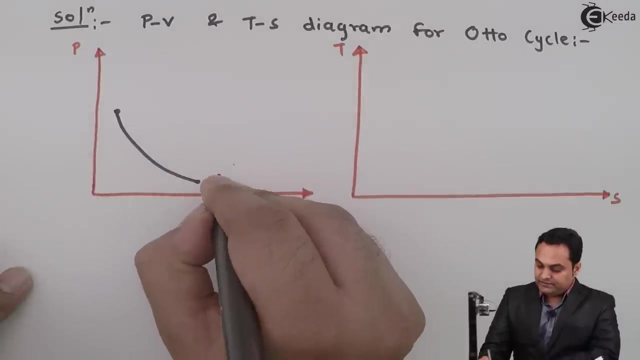 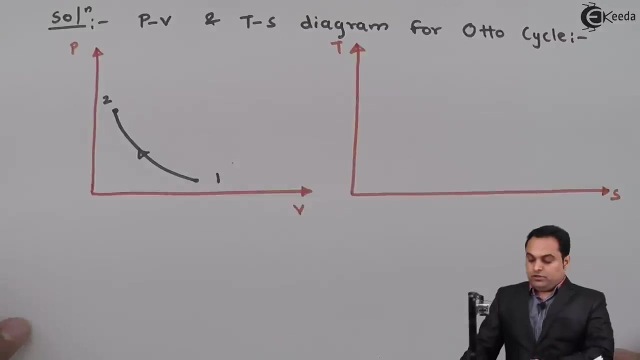 processes. process 1 is called as adiabatic compression, and that adiabatic compression can be shown on pv diagram with the help of a curve. Here, this curve, it indicates process 1 to 2, which is adiabatic compression. Now, in case of adiabatic compression, as it is clear, 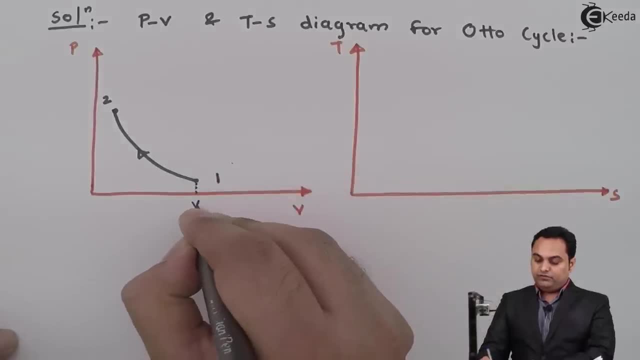 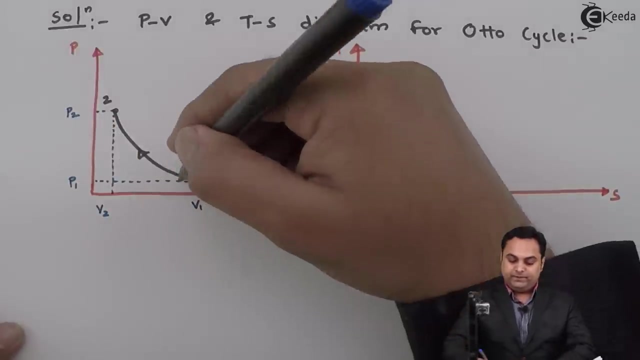 from the diagram: at point 1 the volume is v1. at point 2 the volume is v2.. So from v1 to v2, the volume has decreased, but pressure increases from 0.1- that is, p1- up to p2.. So we have understood that during the adiabatic compression process volume decreases pressure. 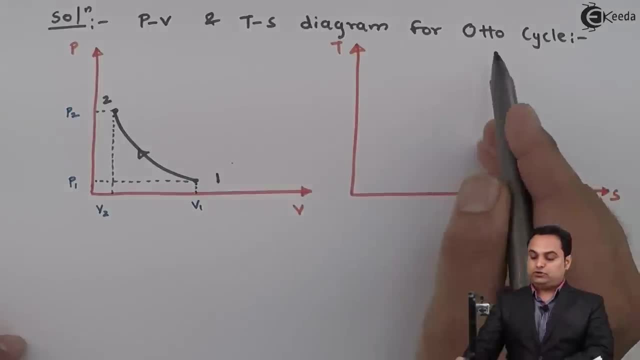 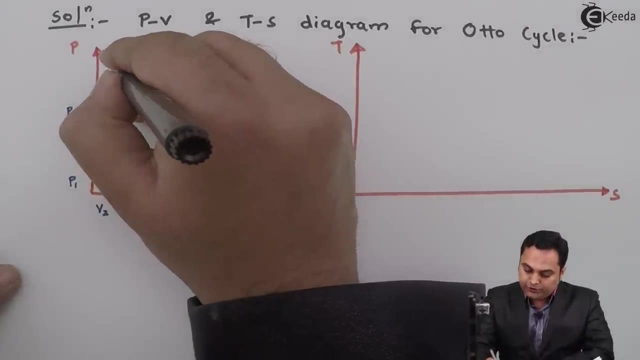 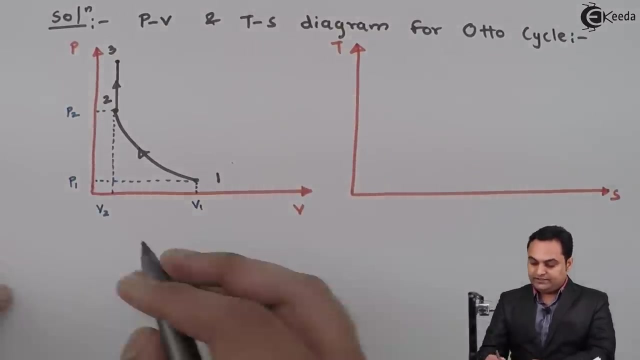 increases. Next, since ah Water cycle is also called as constant volume cycle, the heat will be added at constant volume. So here, from point 2 the heat addition will start and it will be added at constant volume up to point number 3.. So this is the constant volume heat addition. so I can say volume at 2 is equal to volume. 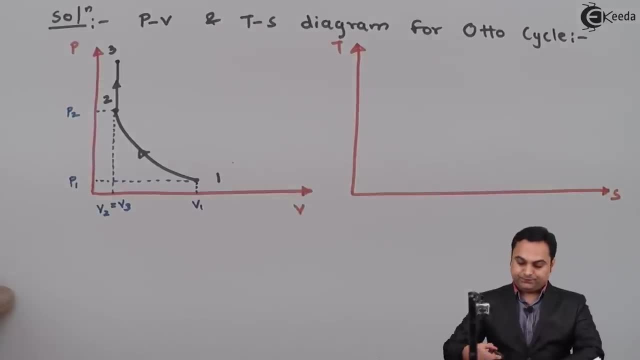 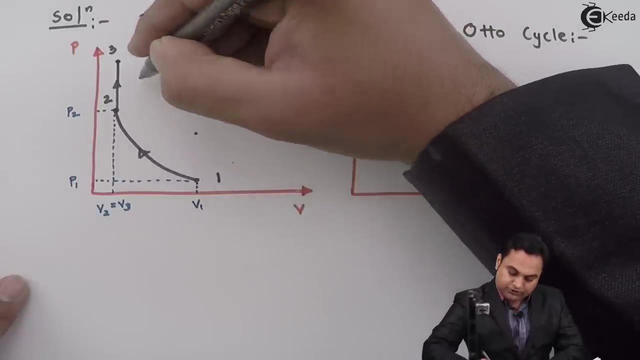 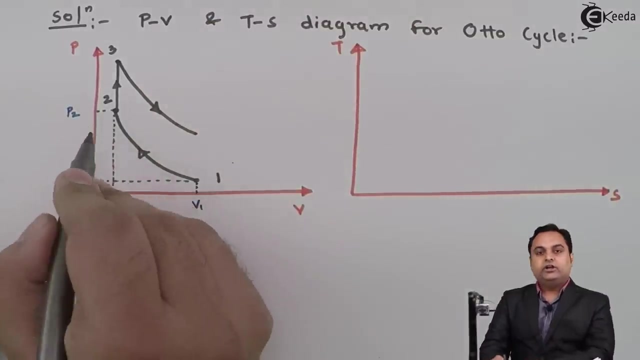 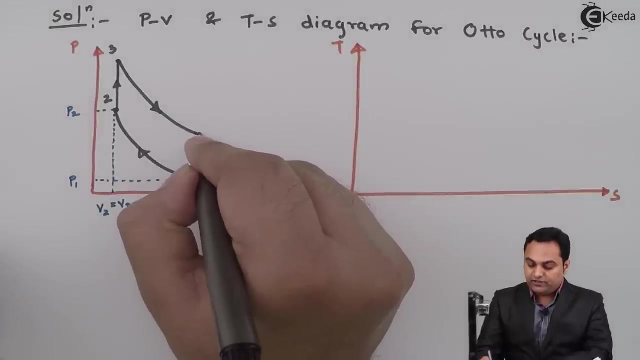 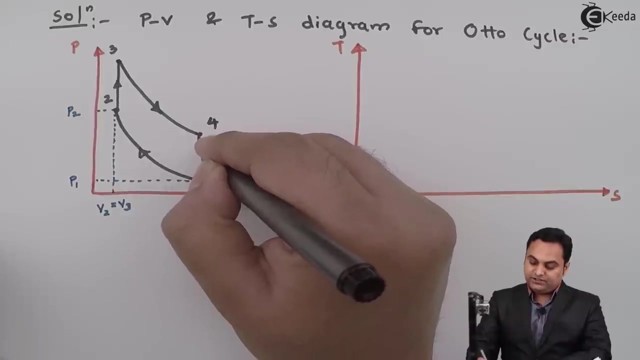 at point 3.. After this there is expansion from point 3 to point 4 and again the expansion, like compression, it was adiabatic or we can say isentropic. similarly, the expansion process is also reversible: adiabatic or we can say isentropic process from 3 to 4. next process, 4 to 1, is heat rejection at 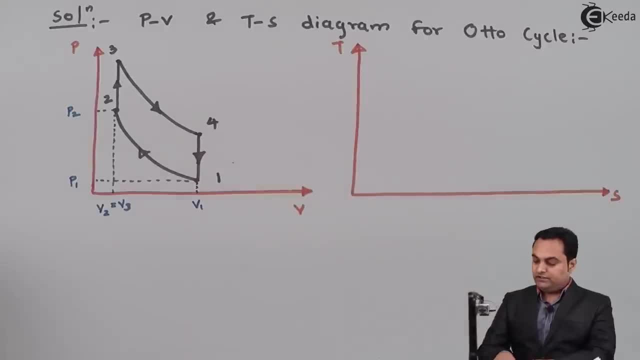 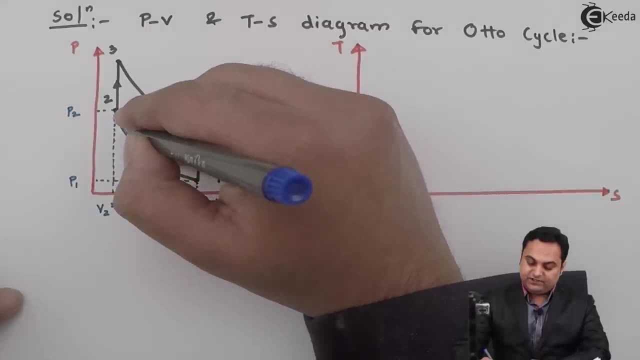 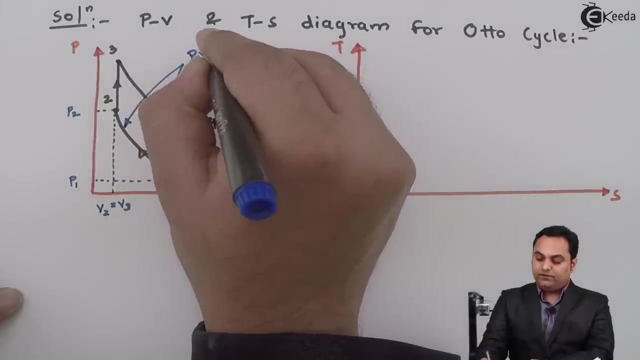 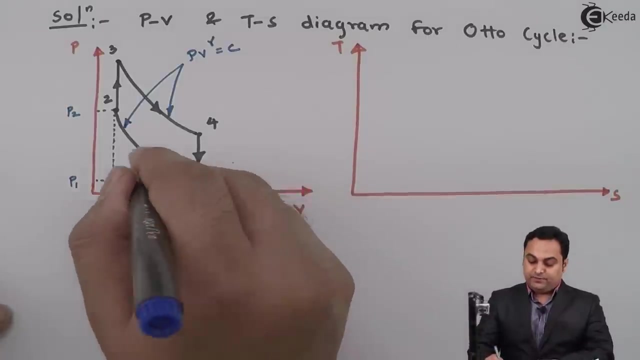 constant volume. so here we can say that v1 is equal to v4. now, during the compression and expansion process, both the law followed is pv raised to gamma is equal to constant. this law is for reversible adiabatic or isentropic process, since the compression and expansion they take place as reversible adiabatic process, so it 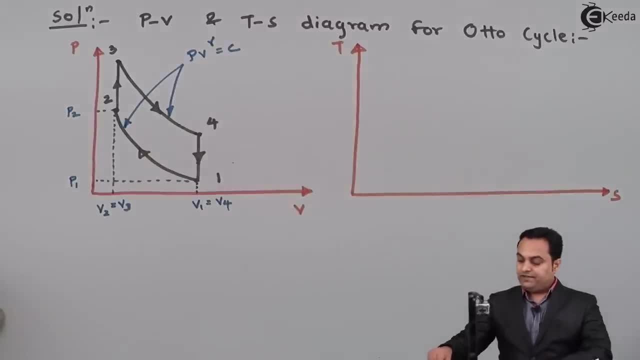 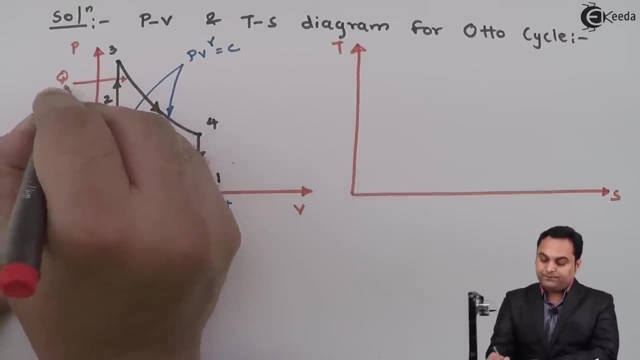 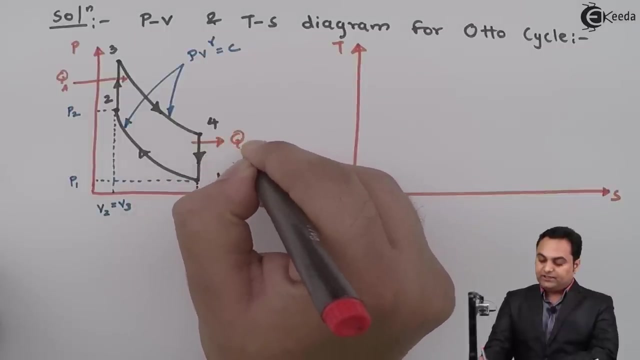 follows the law: pv raised to gamma is equal to constant. next, during process two to three, the heat is added, so i'll write down q suffix a. next, during process four to one, the heat is rejected. so that is q suffix r. now, once i have drawn the pv diagram, next thing would be to draw: 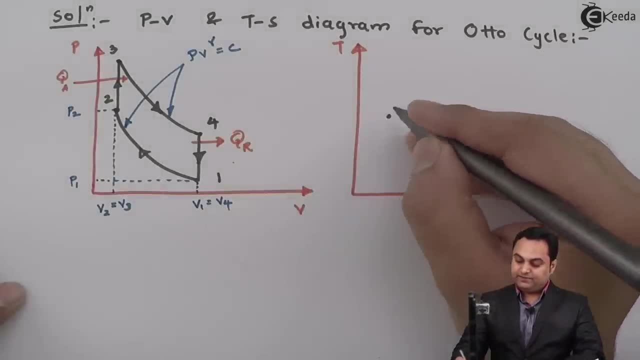 the ts diagram. and in this ts diagram the first process is isentropic compression. so during process one to two entropy will remain constant and during compression process the temperature rises. so, as i can see in the diagram here, s1 is equal to s2, that is the 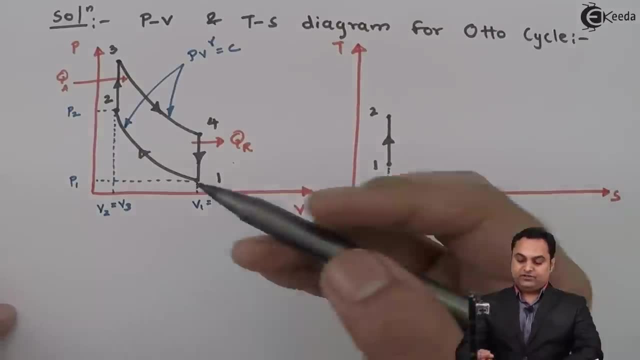 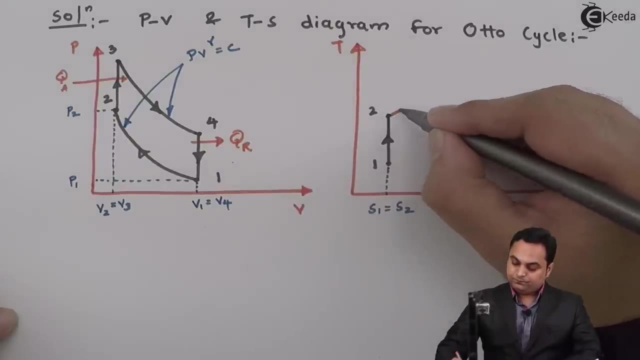 entropy remains constant. next, after that, heat is added, constant volume. so here i am drawing a constant volume line. so over this constant volume line, since heat is added at constant volume. so from point 2 to point 3, the process will follow this constant volume line. here i am getting point three. and since the heat is added, temperature. 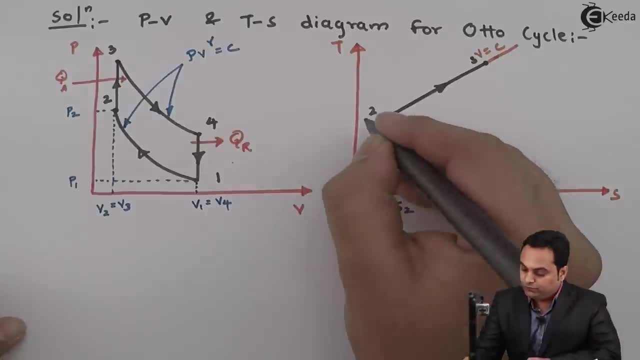 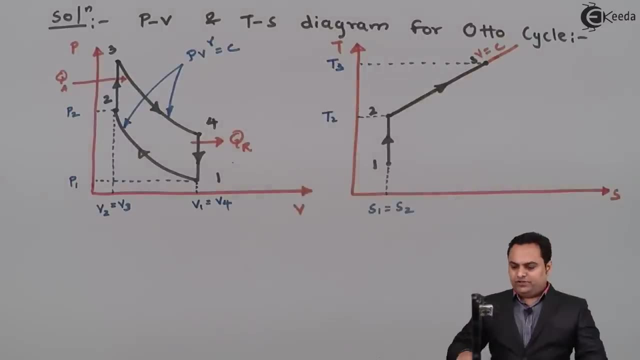 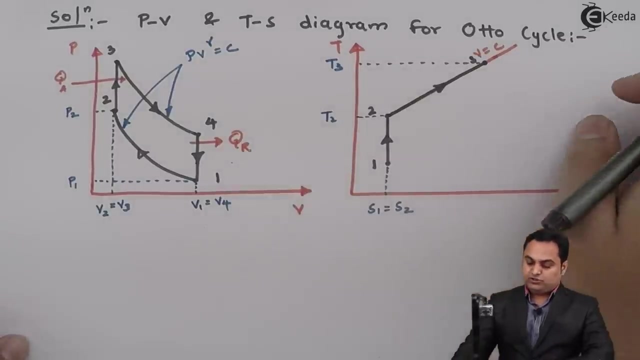 at point 3 is greater than the temperature at point two. so now, here as we are drawing the pv and ts diagram for constant cycle, that is auto cycle process. two to three is constant volume heat addition. three to four was again isentropic expansion. so three to four. 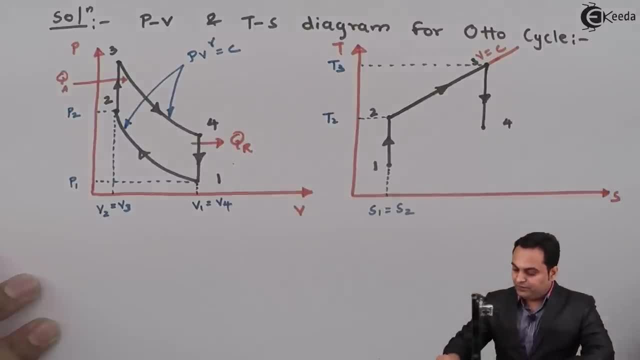 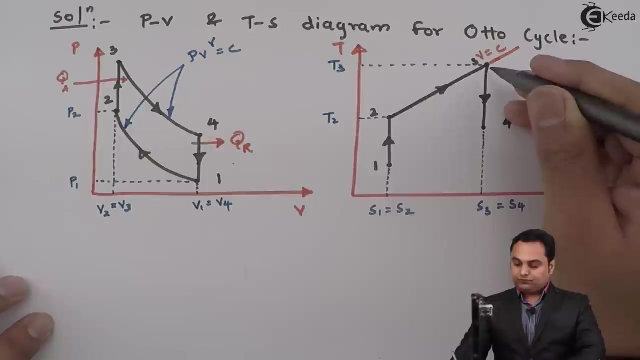 will be isentropic expansion, that is, entropy will remain constant. so i'll write down: s3 is equal to s4, entropy is constant but, as we see, there is drop in temperature from 0.3 to 0.4, so this drop in temperature is utilized to develop some work. 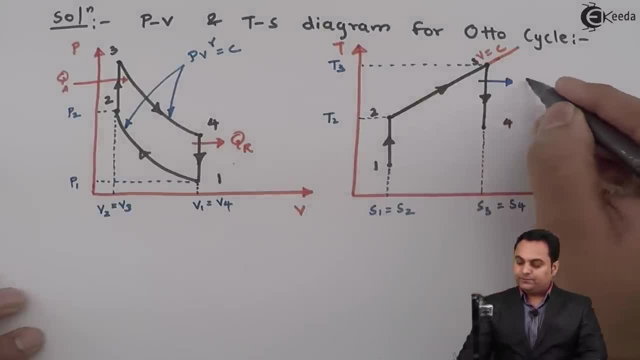 and that work is called as work which we would be getting in the expansion process next, after we have attained the expansion process, then there is heat rejection, which is at constant volume, and for that heat rejection, again, i'll draw a constant volume line, and since heat is rejected from 0.4 to 1, so heat will be rejected here. 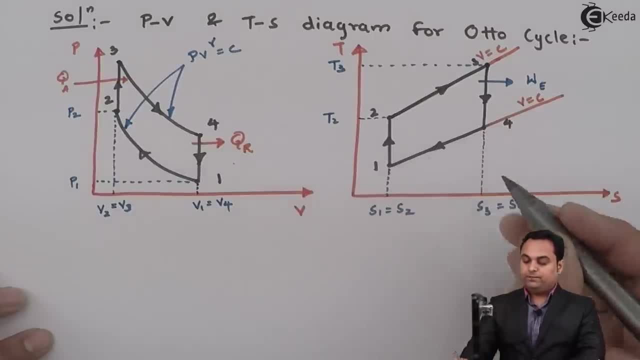 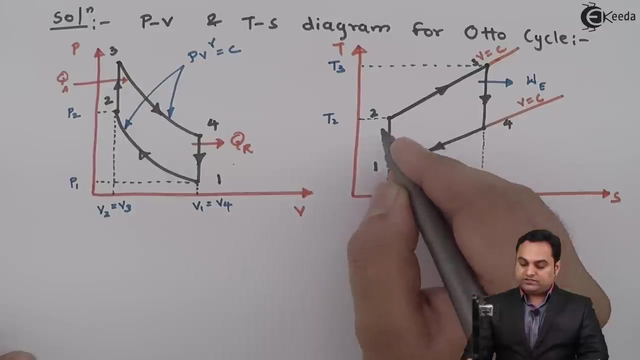 from 0.4 to 1 and again it follows a constant volume line, that is, volume of 0.1 and 0.4. they are same as previously. volume lines of 2 and 3. they were same now during 1 to 2. the work is done. 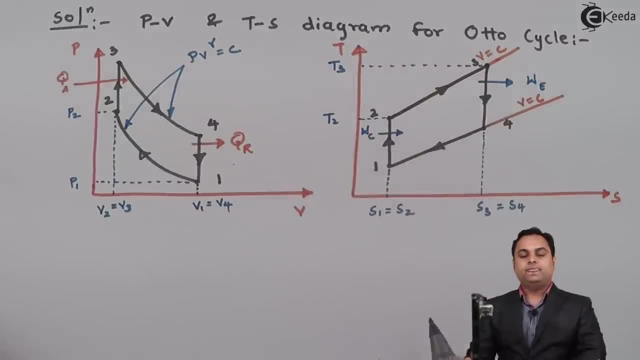 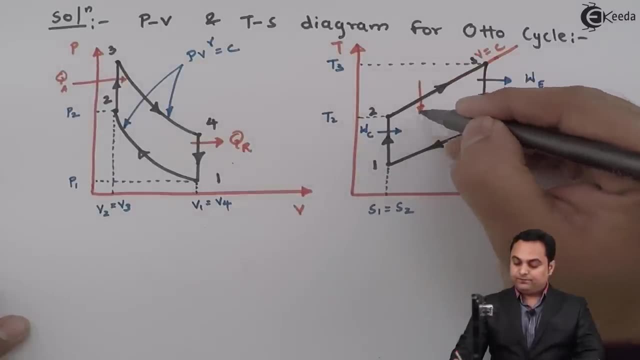 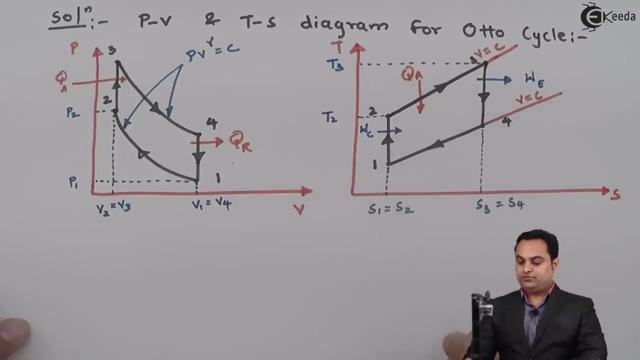 during compression, or we can say the work is done on the air during compression process. next, from 2 to 3, the heat has been added, so this will become qa for process. three to four there is work which we are getting in expansion process, and four to one is the heat which is rejected out of the system. 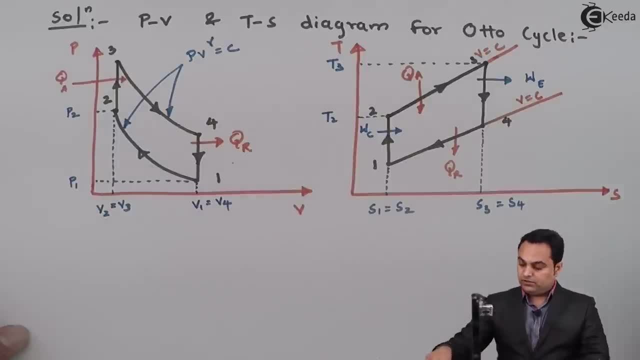 so similarly, i can mark here on the pv diagram that during one to two the work is done in compression and from three to four the work we are getting in expansion. now, once we have drawn the pv and th diagram, i can explain it again that what we have to calculate here, the first thing is compression. 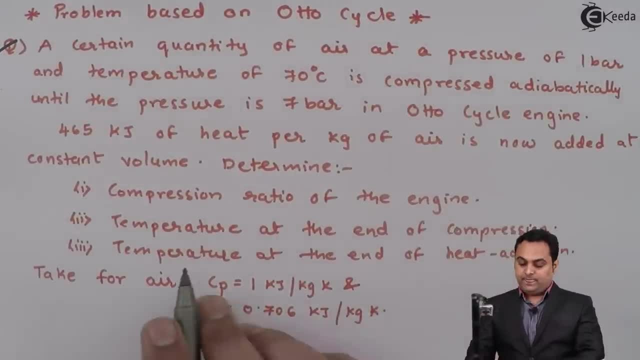 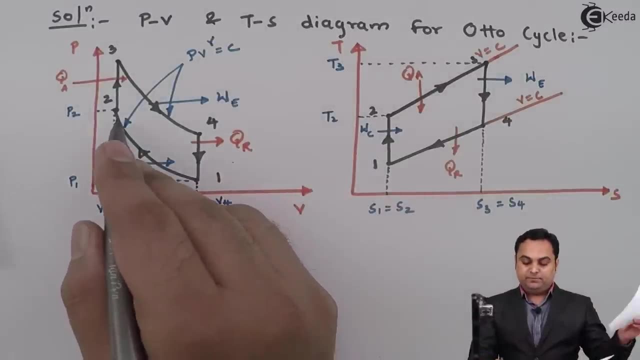 ratio of the engine, which is denoted as r suffix c. next is temperature at the end of compression. so So, if we see, compression starts from point number 1 and it gets completed at point number 2.. So temperature at the end of compression means we have to find out the value of T2.. 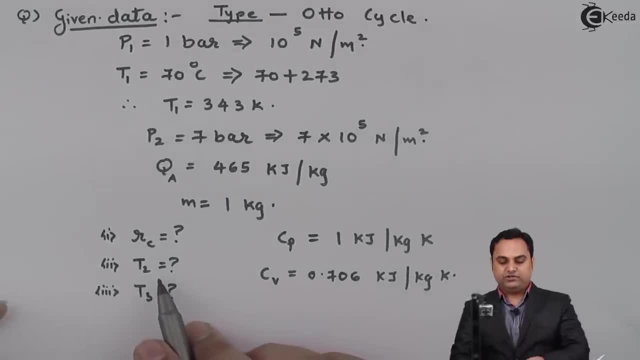 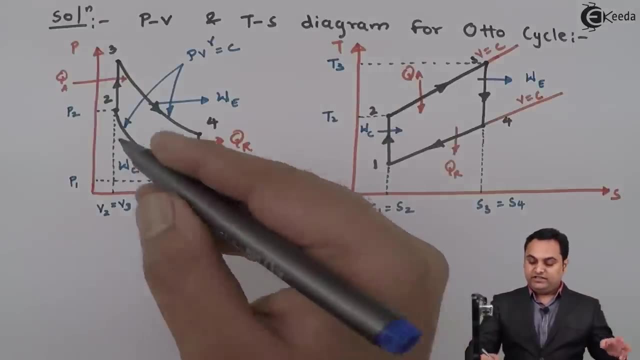 So, as I have written in the data, we have to find out T2 as the second question And then the third question is temperature at the end of heat addition. Now we see that heat addition at constant volume. it starts at point number 2 and finishes at point number 3.. 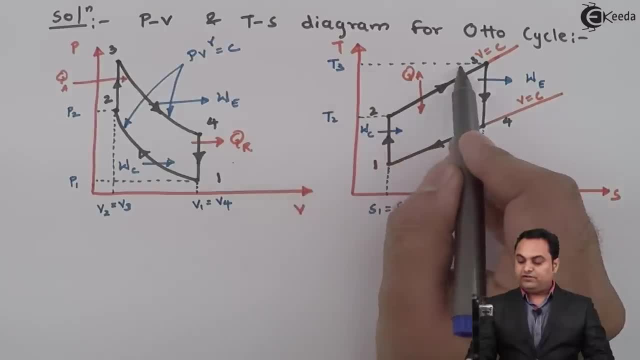 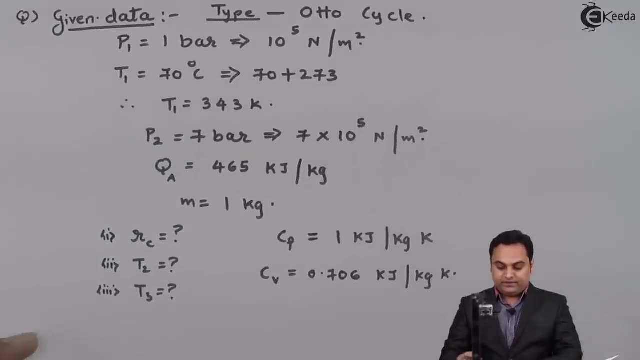 So temperature at the end of heat addition means we have to calculate the value of T3.. So here we have understood that how many unknowns are there and what we have to calculate from them. So first I will start with the calculation of RC, which is called as compression ratio. 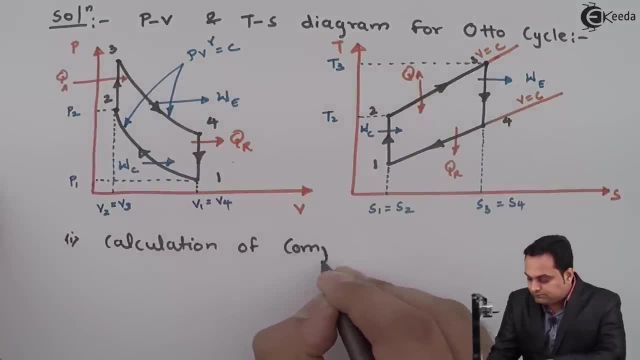 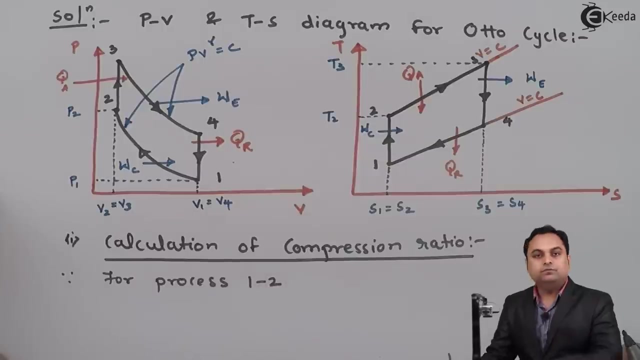 So it is calculation of compression ratio. So now I will write down that, since for process 1 to 2, which is also called as isentropic process, Here the relation can be written as T2 upon T1, that is, higher temperature upon lower temperature. 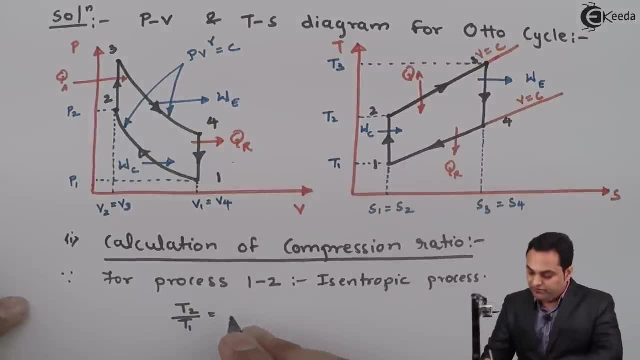 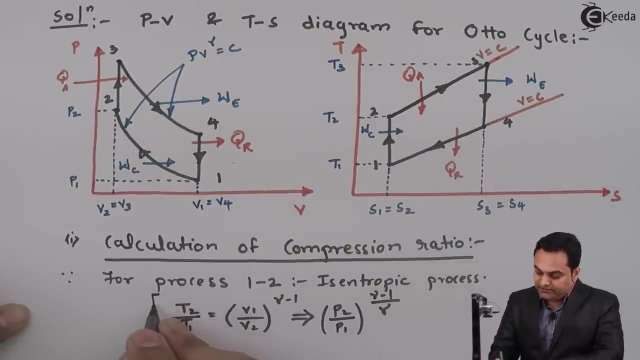 Is equal to V1 by V2 raise to gamma minus 1, and this is also equal to P2 by P1 raise to gamma minus 1 upon gamma. This is the relation of isentropic process and after writing this relation, this was the relation. 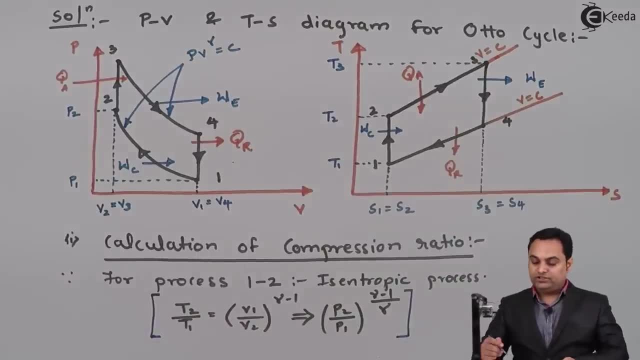 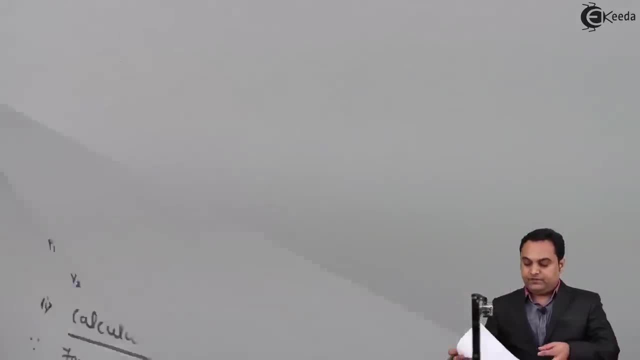 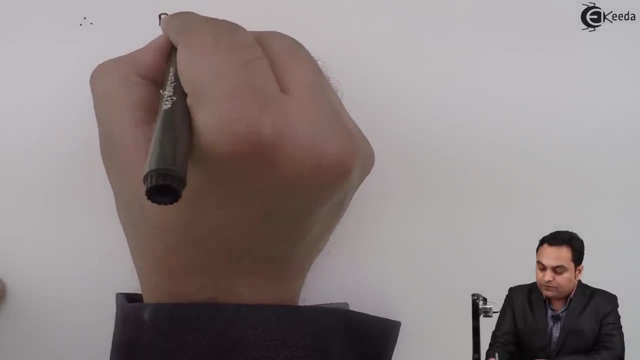 Between temperature, volume and pressure. Now I will write one more relation which is related to PV. raise to gamma is equal to constant for state 1 and 2.. I will write down that after this, therefore, P1- V1 raise to gamma is equal to P2- V2 raise to gamma. 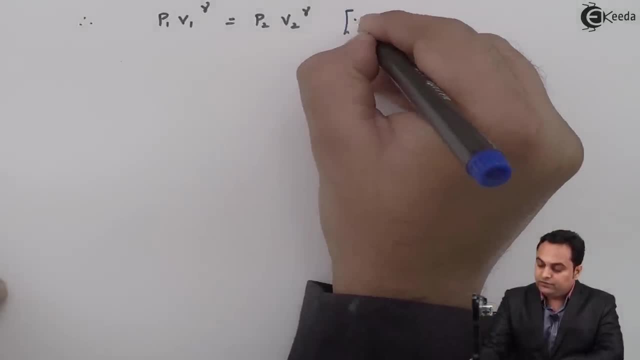 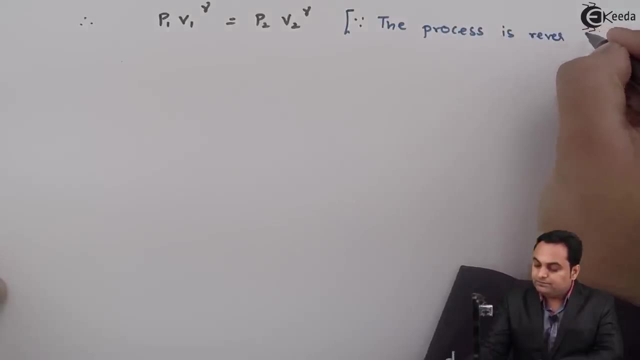 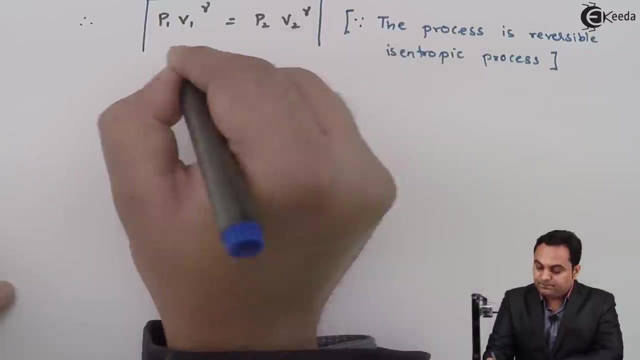 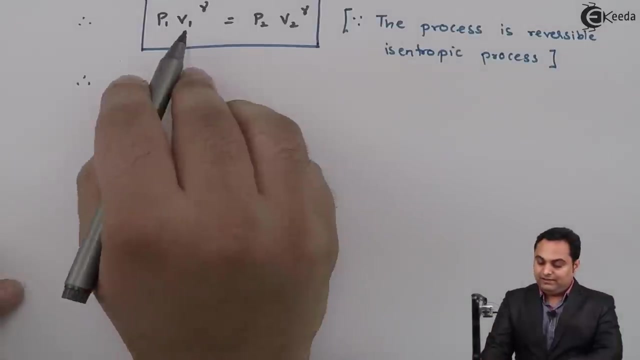 This we are writing since the process Okay, Okay, So this is reversible isentropic process. So now I will utilize this relation. So therefore here I will write it in a special form that is P2.. I will shift P1 here. 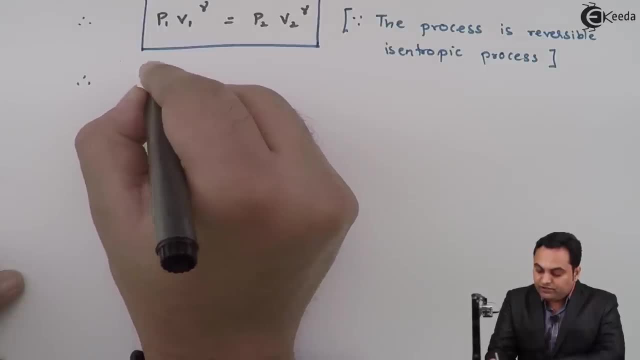 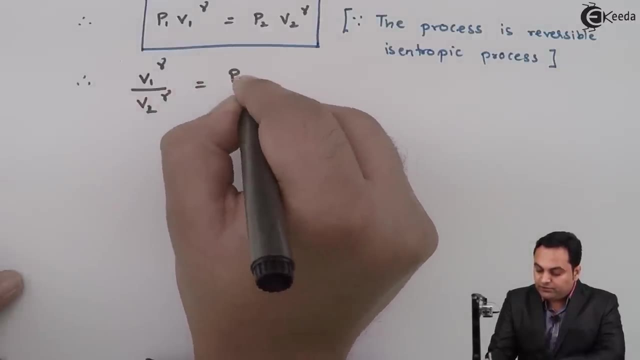 So it will be Here. Here we are left, with V1 raise to gamma and V2 raise to gamma. I will bring it on to the left hand side. Here we have P2.. This P1 will go into the denominator. 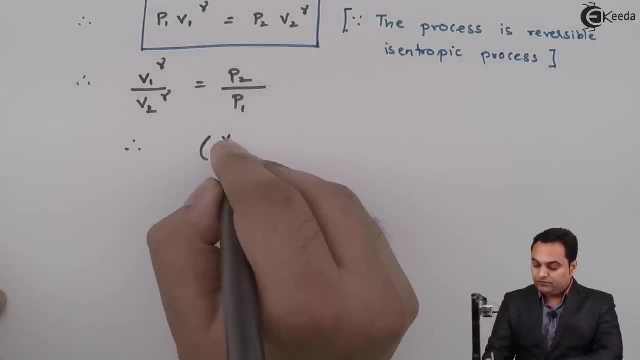 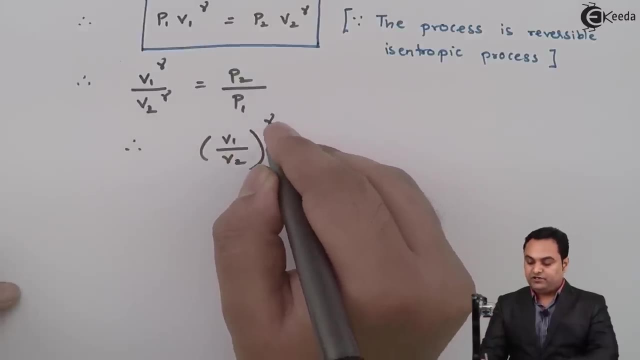 So after this, therefore, V1 by V2.. This gamma, I can take it as common. So it is common raise to power gamma equal to P2 by P1.. Now, P2 by P1. If I see in the data, 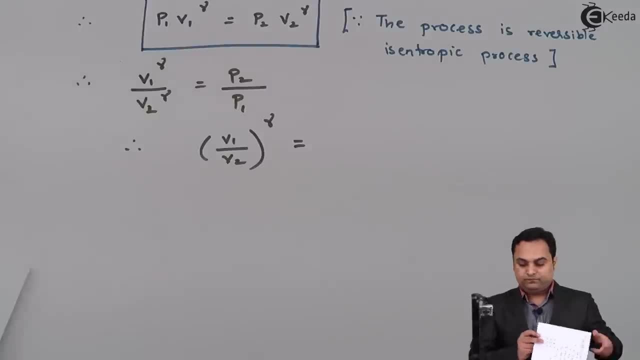 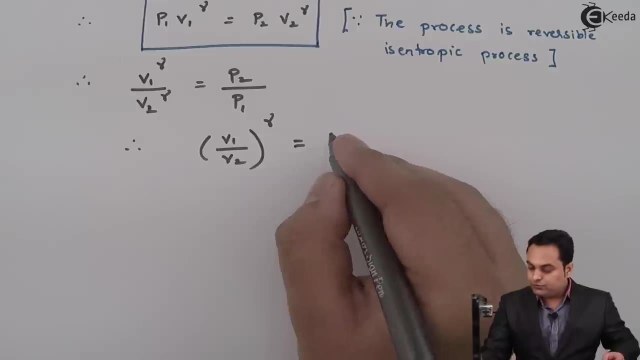 So P2 and P1 values are given. that is, P2 is equal to 7 bar, P1 is equal to 1 bar. So 7 into 10 raise to 5.. I am writing it in terms of Newton per meter square. 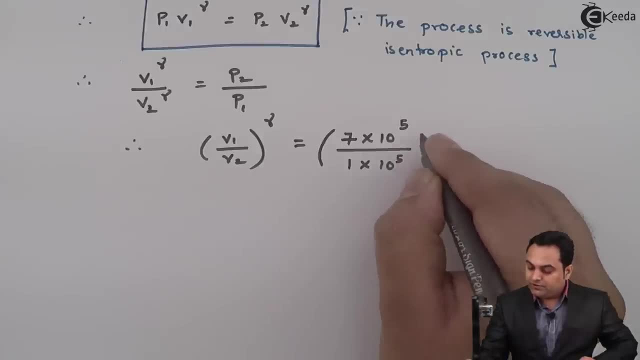 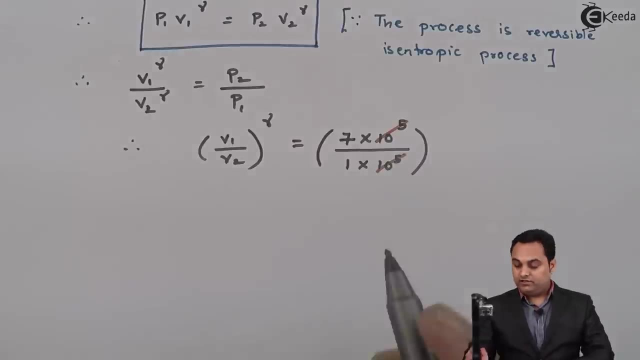 Again, P1 is 1 into 10 raise to 5 Newton per meter square, 10 raise to 5, 10 raise to 5 will get cancelled out. So it means If If we are writing the pressure ratio, then we can directly write it in terms of bar, because 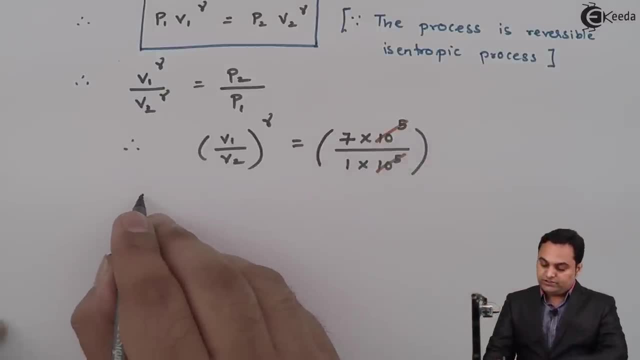 in terms of Newton per meter square. it will get cancelled out Next. therefore, V1 by V2 is nothing, but it is called as compression ratio. RC is equal to now. here we have 7 upon 1, which is 7. raise to the power. 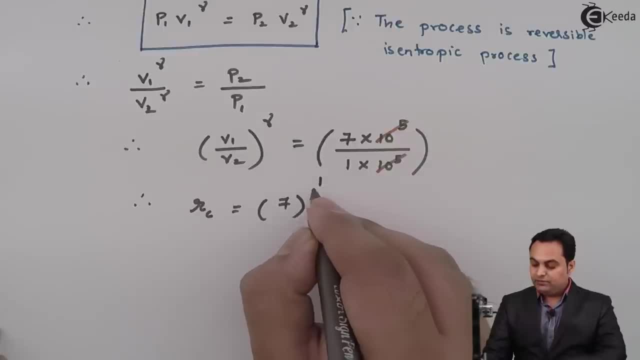 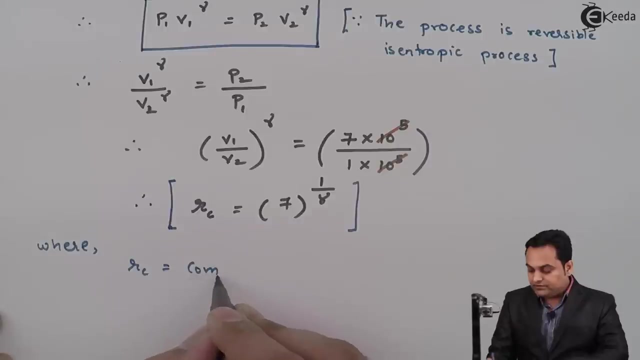 Now this gamma. when it goes on to the other side, it would become 1 upon gamma. Now, after writing this, I will say that where R suffix C, it is called as compression ratio and it is equal to cylinder volume upon clearance volume. So therefore RC can be written as: 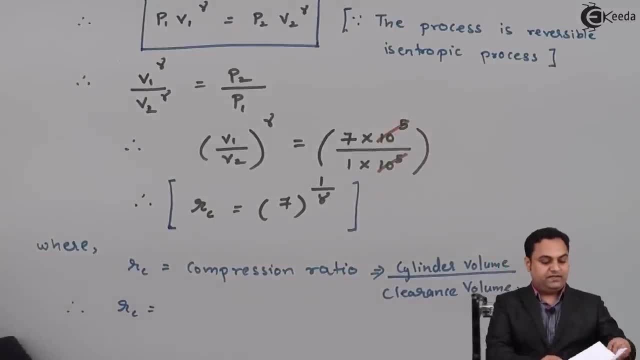 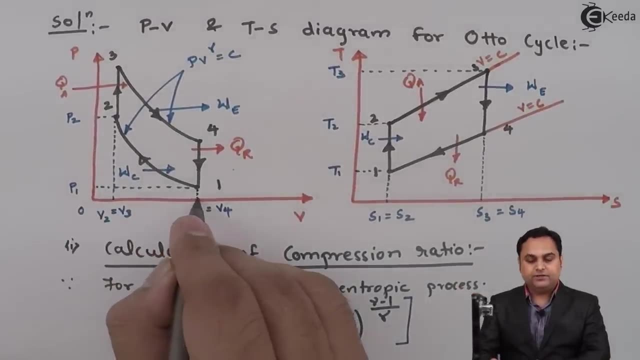 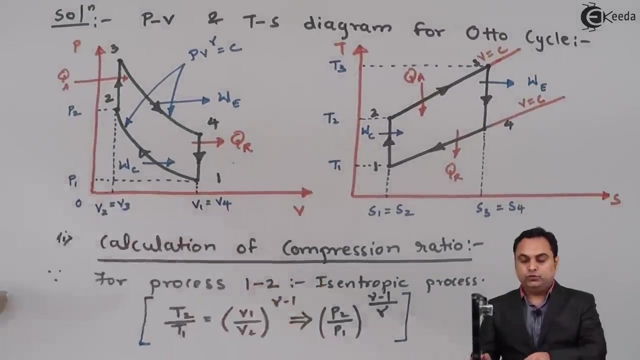 Yes, Yes, Yes, Yes. Now from the PV diagram It is clear that V1 is the volume of the cylinder cylinder volume. So V1 clearance volume is only up to 0.2.. So V2 is a clearance volume. 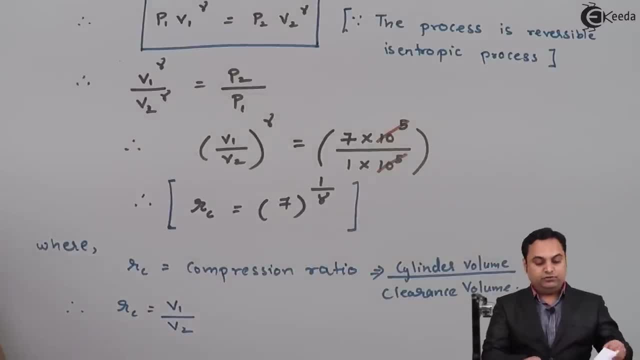 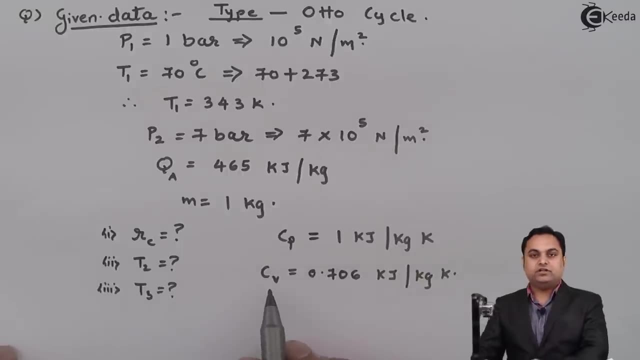 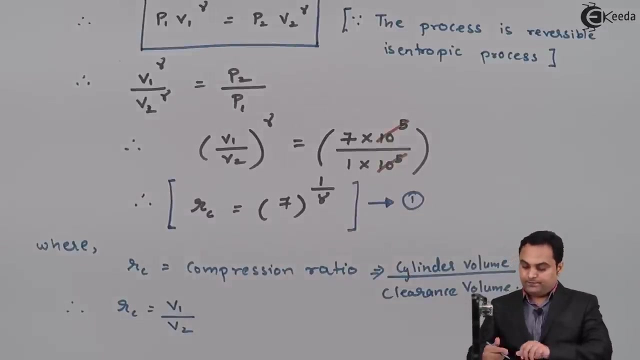 So V1 by V2 is RC. now this gamma value we do not have. It is not given in the data, But CP and CV values are given. So keeping this as equation number one and I'll go for the calculation of gamma. so 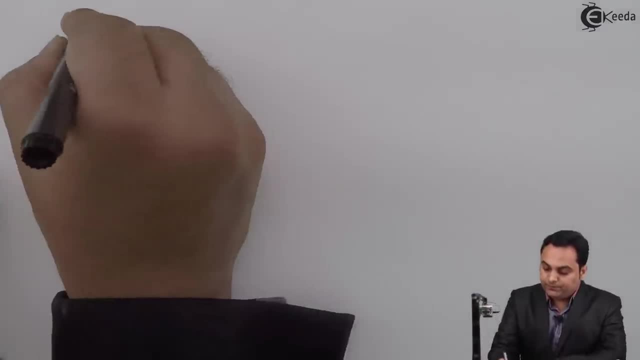 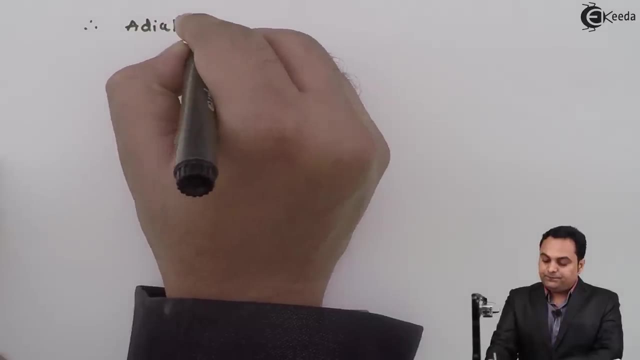 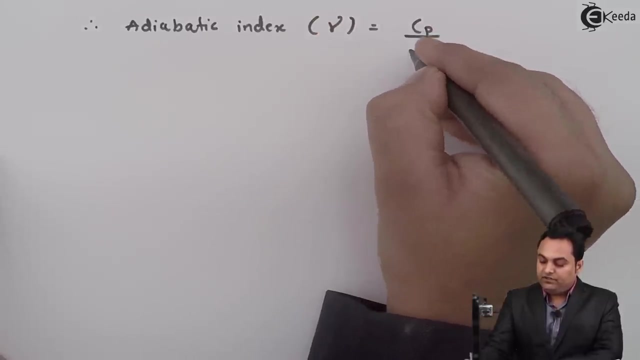 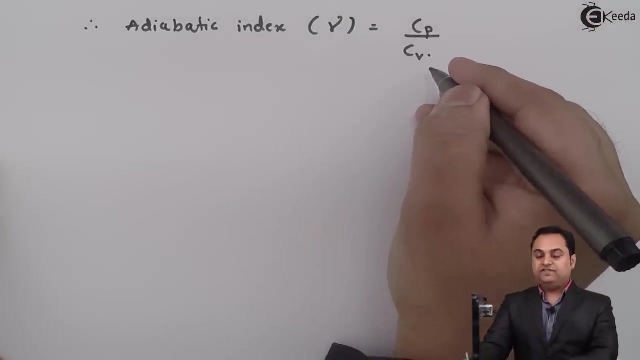 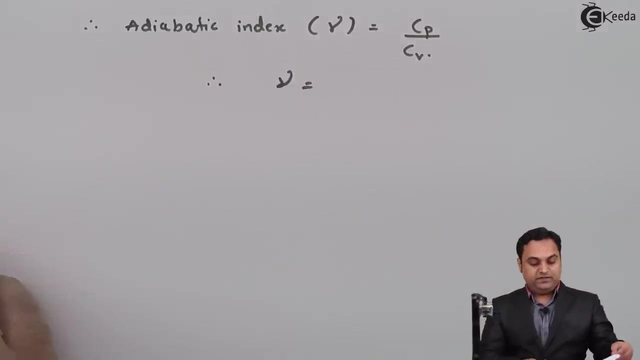 after reaching this stage. I'll say that therefore gamma it is called as adiabatic index. so adiabatic index gamma is equal to CP upon CV. that is the relation of gamma. CP is specific heated constant volume, constant pressure, CV is specific heated constant volume. so therefore gamma will become now CP is. 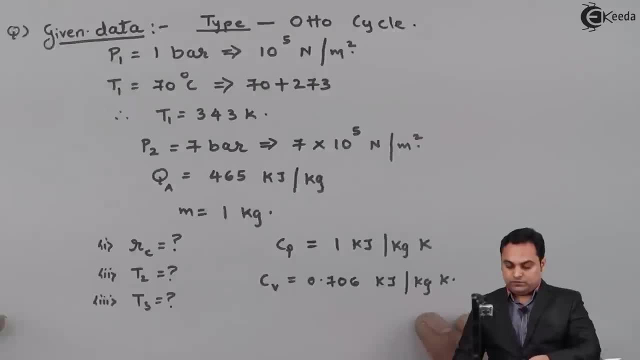 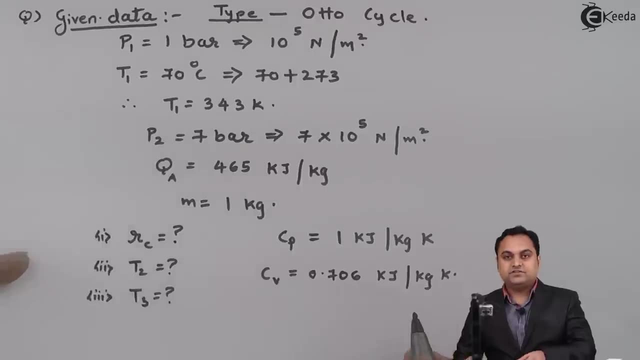 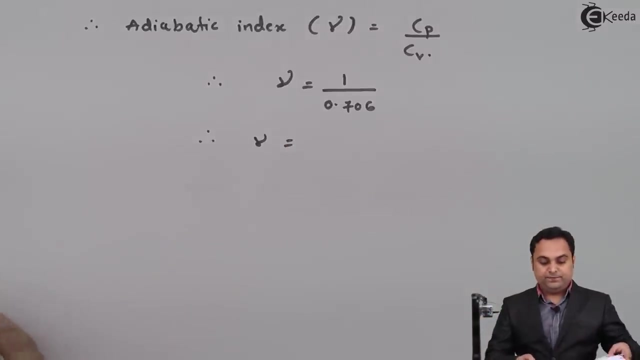 given it is 1 kilojoule per kg Kelvin, CV 0.706. so therefore, gamma value it. it comes out to be 1.41. now, after getting this gamma value, I will put it in equation number 1, where in we will be getting the value of RC. so I will write down: therefore, put gamma. 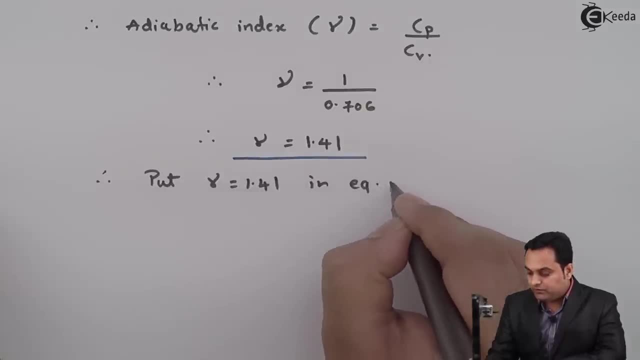 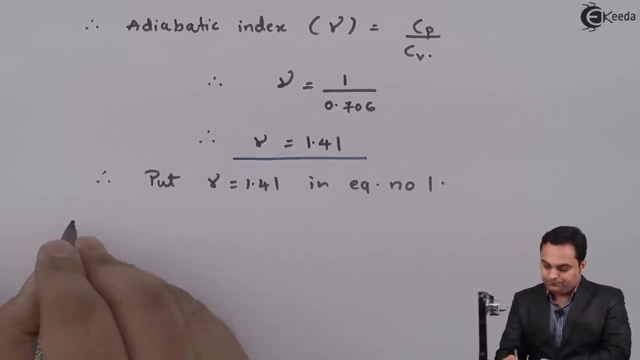 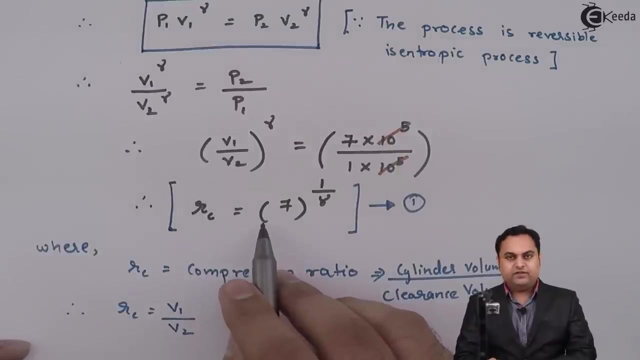 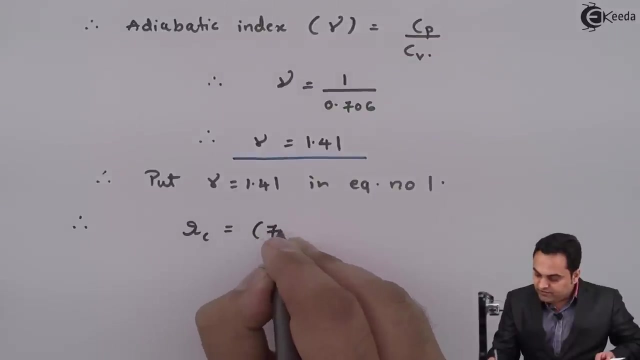 is equal to 1.41 in equation number 1. so now here I am putting: gamma is equal to 1.41 in equation number 1. therefore in equation 1 we had R suffix. t is equal to 7, raise to the power 1 upon gamma. so that will be R suffix. c is equal to 7, raise to the power, now 1 upon. 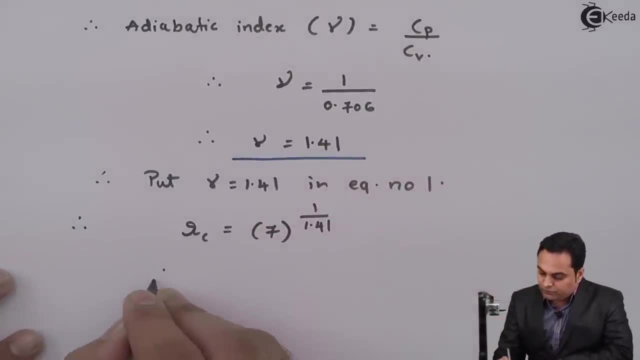 gamma. gamma is 1.41.. So from this I will get the value of RC on the calculation and my answer is 3.975.. So here is the first answer, that is, we have calculated the value of compression ratio. now, after the compression ratio, the next question was: 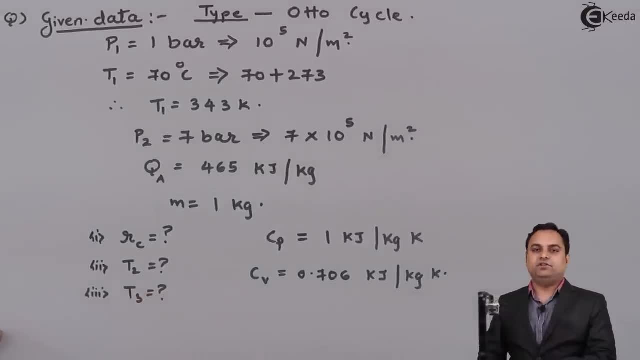 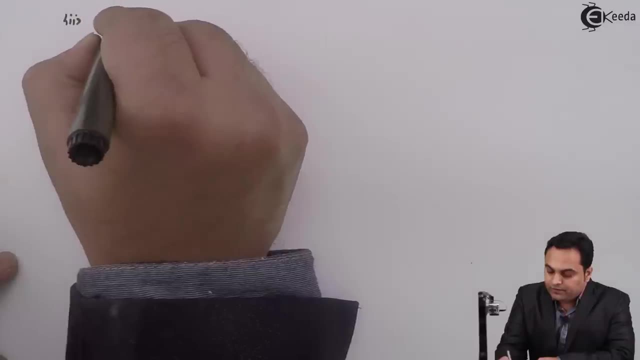 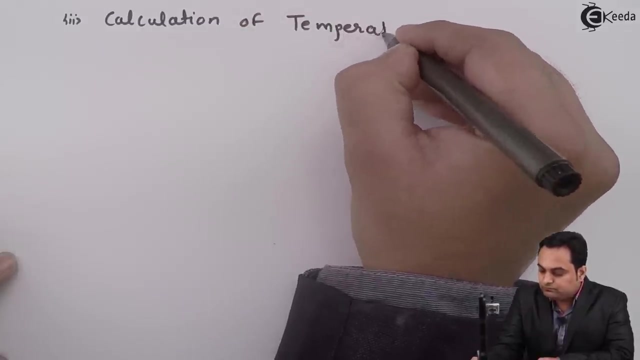 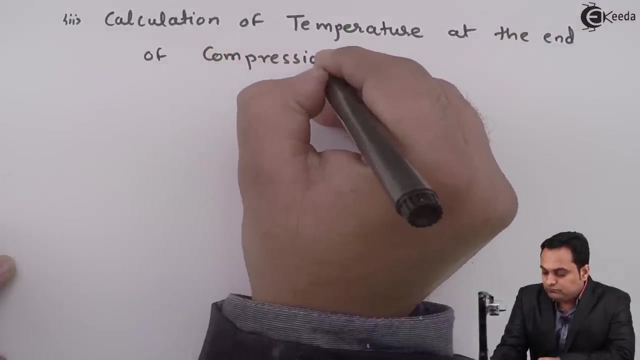 to get the value of T2, that is, the temperature after compression. so ok, here I saved the value of T2. Okay. so here is the thing: when we take the value of T2, if we take it from the ratio of T2 to k times the elevation, or this is the number here: 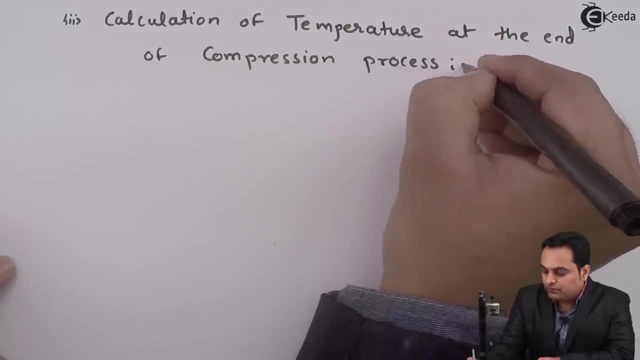 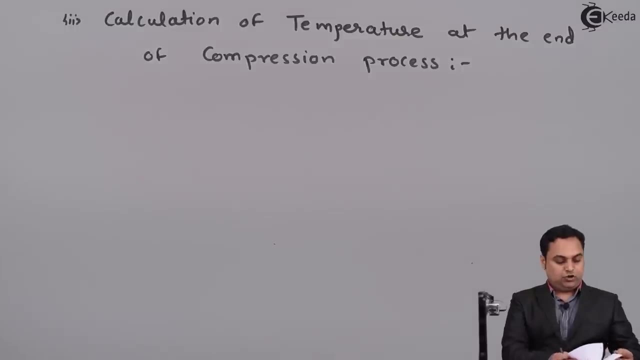 here we have right, right, and luckily for this we now have selected at equal to T d, which is equal to k times v. everything else we have to do is to calculate the undo, that is, k times v, which is equal to 3.75 to k times V. 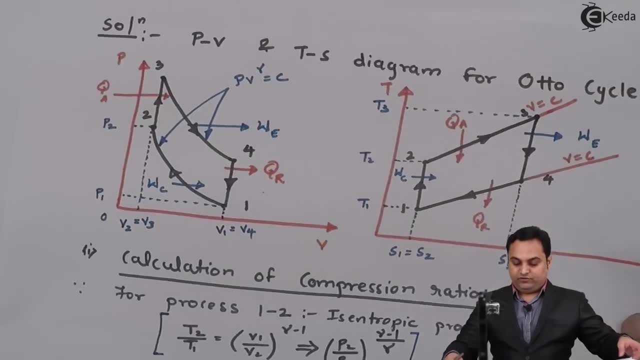 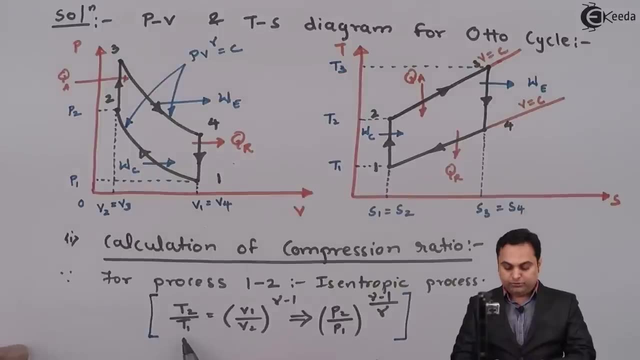 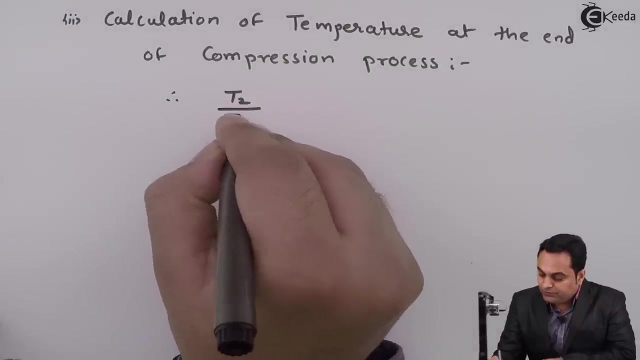 So we prepare this variable or we can say reversible adiabatic, and for reversible adiabatic compression we can use this relation, that is previously, which I have written for process 1 to 2. now T2 by T1 can be written as V1 by V2 raise to gamma minus 1. so therefore T2 by T1 is equal to V1 by. 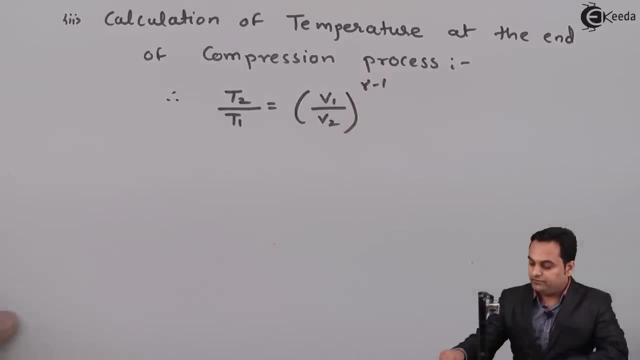 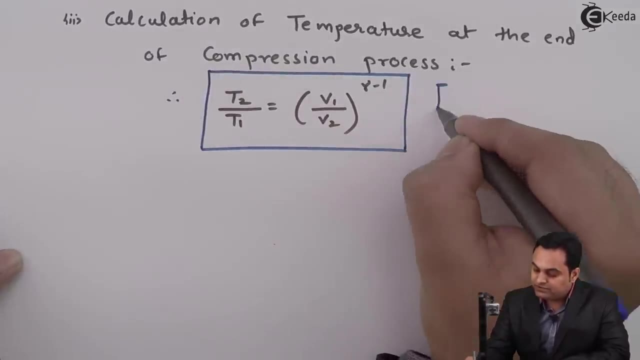 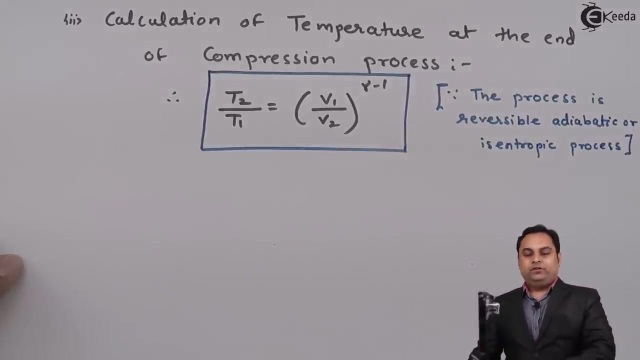 V2 raise to gamma minus 1, and this relation is for, since the process is reversible, adiabatic or isentropic process. Now, after writing this relation, I will say that therefore, T2 by T1 is equal to V1 by V2 is nothing, it is called as RC, that is compression ratio, and that compression ratio value is 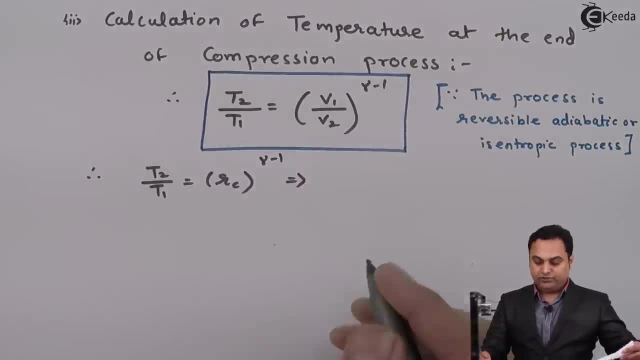 we have found out it was 3.975. that was our first answer. raise to gamma, which was 1.41 minus 1. so therefore T2 by T1 is equal to V1 by V2 is nothing. it is called as RC. that is compression ratio. 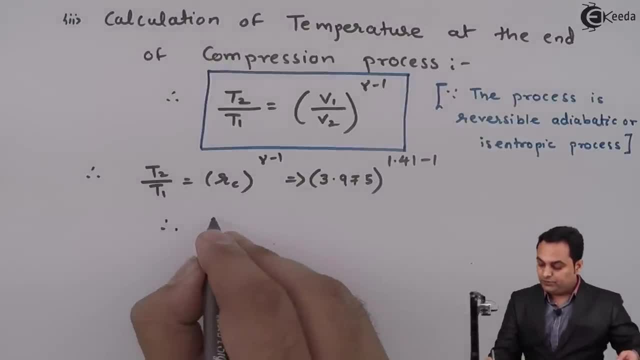 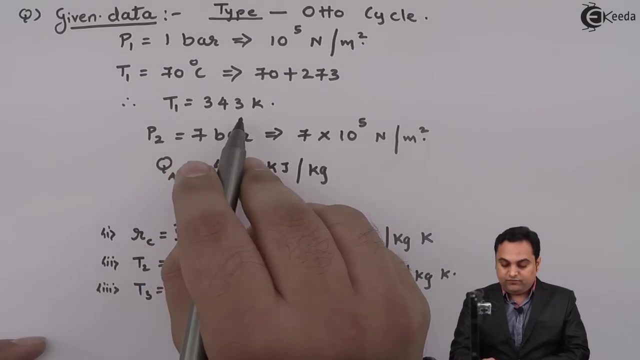 here I will get it, as T2 by T1 is equal to this. complete value is 1.76. so T2, this T1, I will send on to the other side, and the value of T1 is 343, so 343 will be multiplied here. 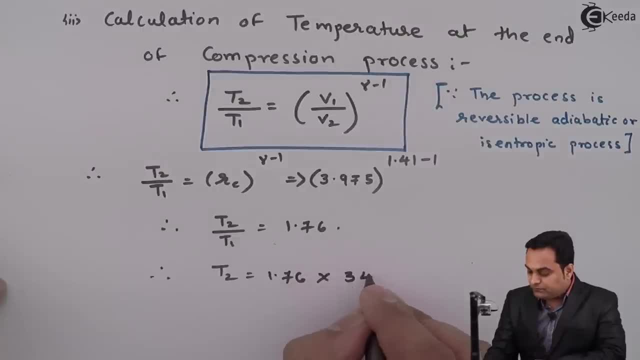 that is 1.76 into 343 and hence the answer T2 comes out to be 1.76.. So this is the temperature at the end of compression process and our answer number. second, after reaching here, the last question was to calculate the temperature at the end. 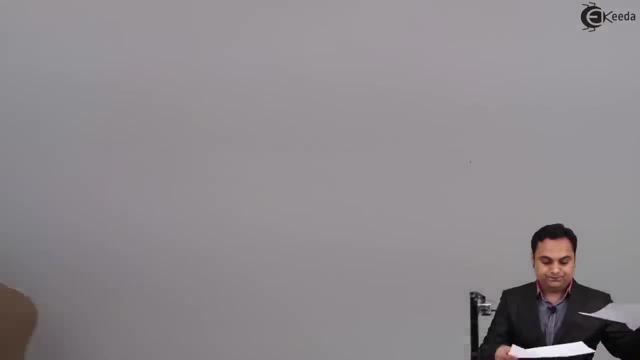 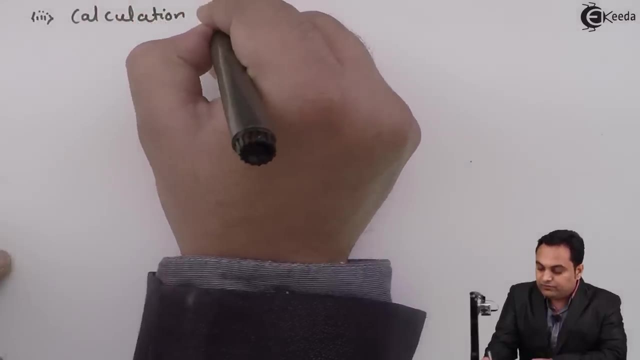 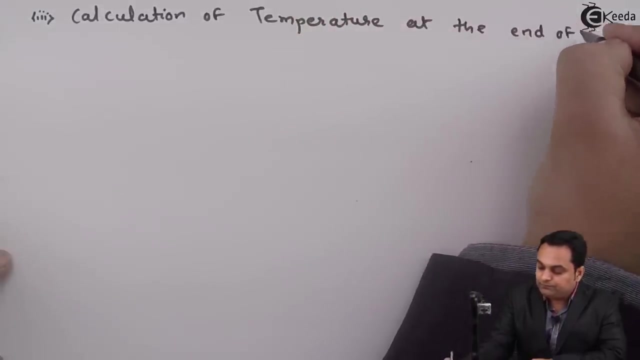 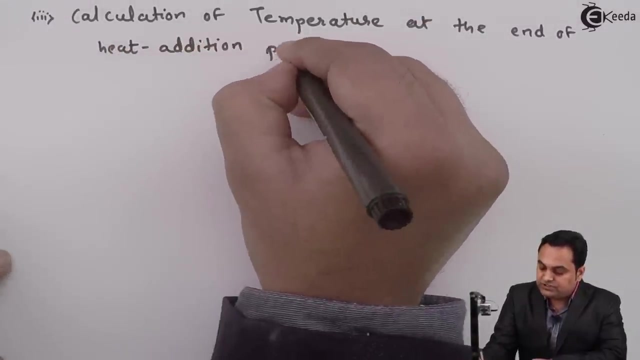 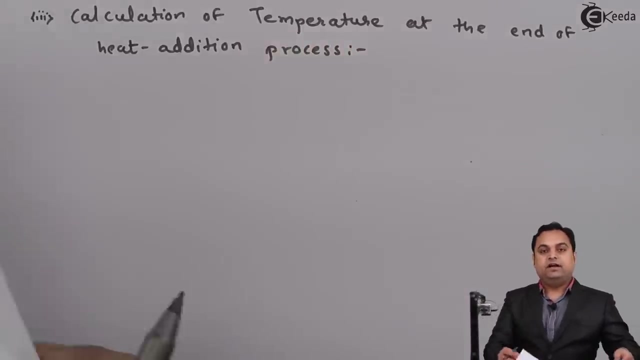 of heat addition which is T3. So calculation of T2 by T1.. So I will calculate the temperature at the end of heat addition process. so now, to calculate the temperature at the end of heat addition process, I will utilize the heat added which is given in the problem. 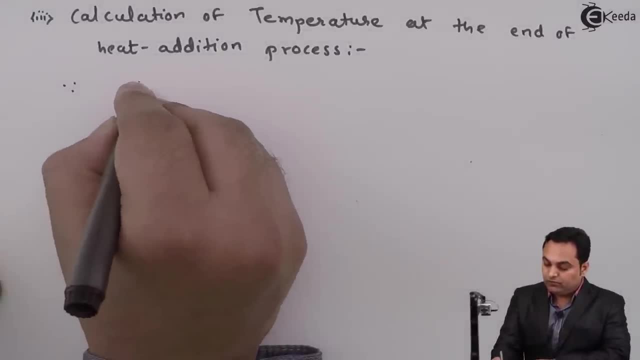 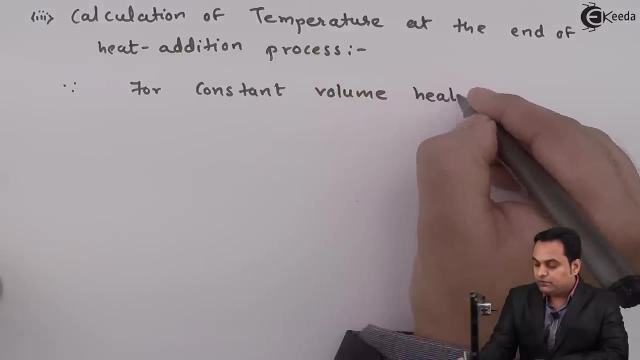 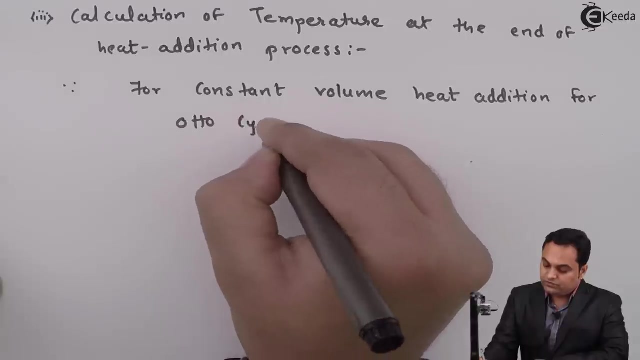 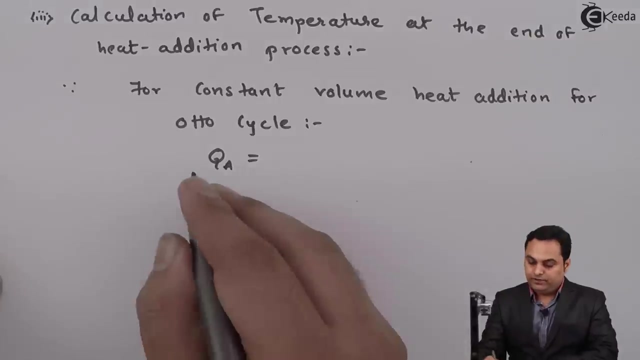 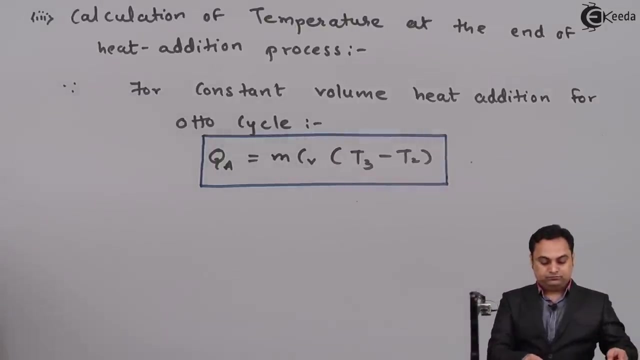 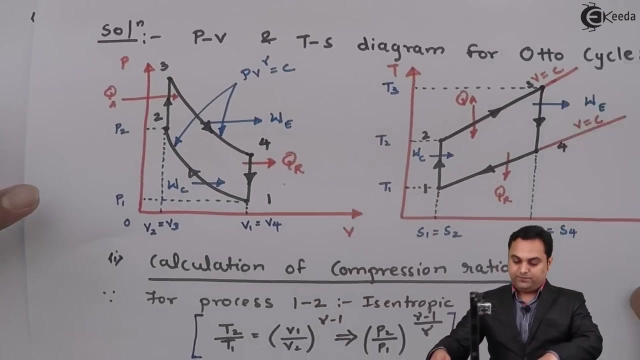 I will say that since For constant volume heat addition for auto cycle I can write down QA that is, heat added at constant volume is equal to MCV into T3 minus T2.. This can be explained from the TV. it is PV and TS diagram. here heat is added at constant.